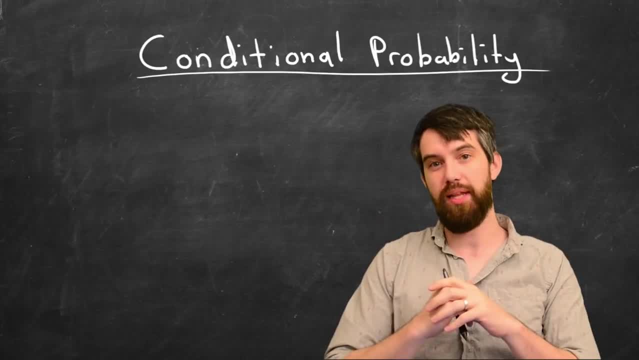 In this video, we're going to talk about something called conditional probability. The idea with a conditional probability is that we want to figure out the probability of something, given that we have some other piece of information, some other piece of information that we can bring to the 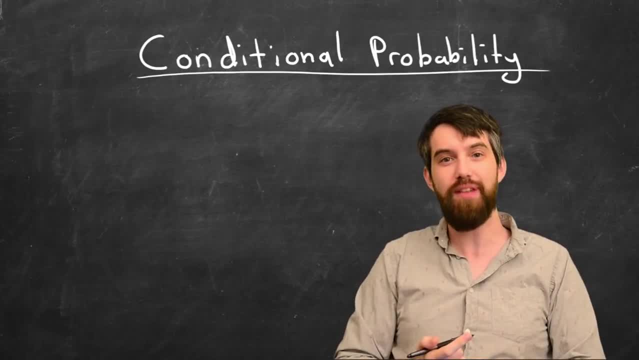 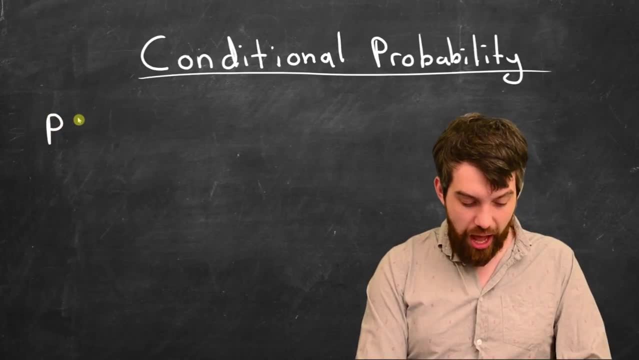 table that will influence the probability of whatever it is that we're investigating Now. the way we write this down is with the following notation: We're going to refer to the probability of A given B, So this vertical bar that we have here is is referred to as or. 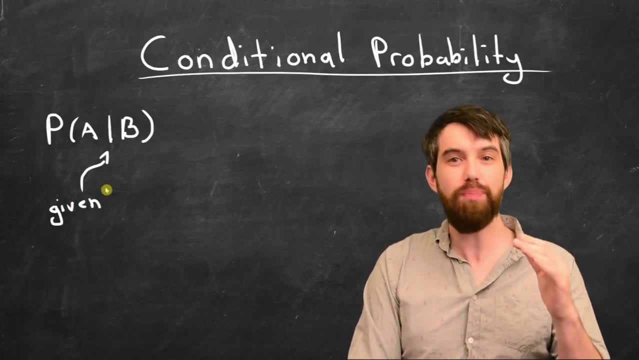 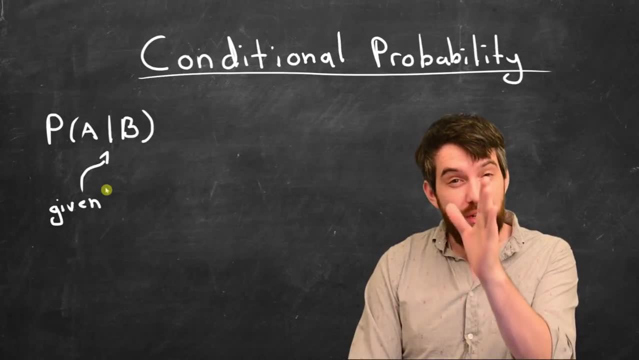 read off as given and what it means is: this is the probability of A, the thing I want, the thing I'm investigating, the probability of some event A, given that I have this other piece of information, given that I know that this event B has occurred. 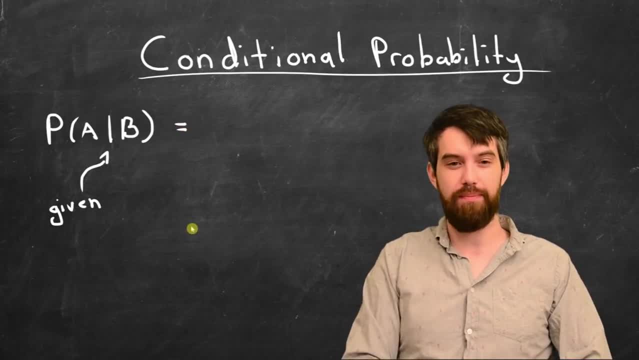 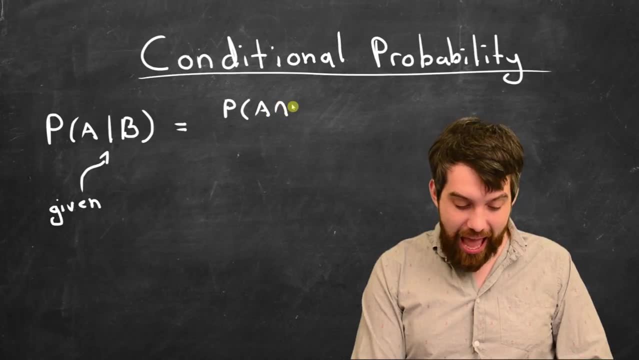 So we want to have some formula for how we're going to compute this. It is a quotient of two. It is the probability that we have both the event A and the event B. So I write this as an intersection. It means the probability of A. 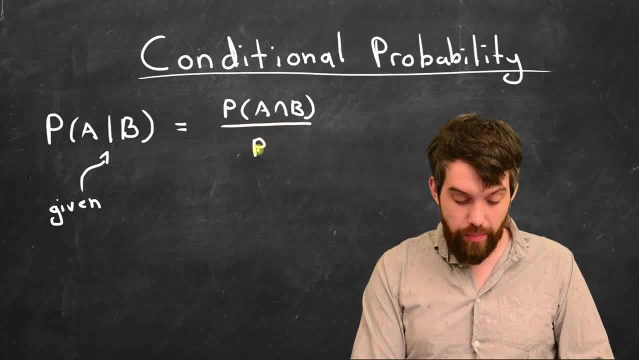 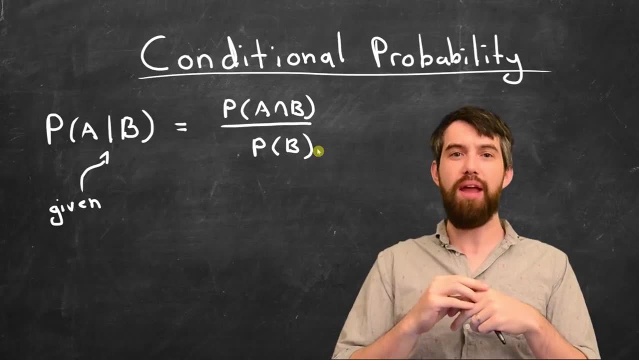 and B all divided out by the probability just of B. Now the way I like to think about this formula is that we're looking not at all possible events. We're looking at this, the sort of narrowed sample space of knowing that this event B has occurred, and we're asking: well, what's the probability? 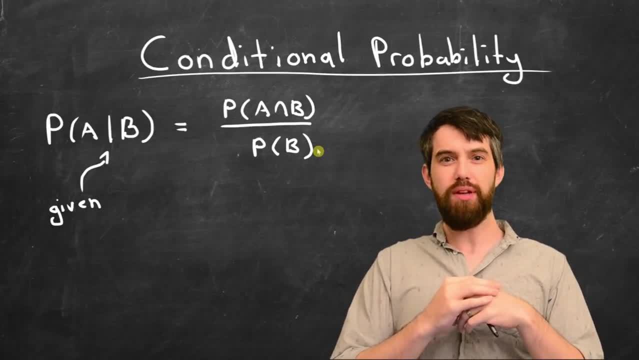 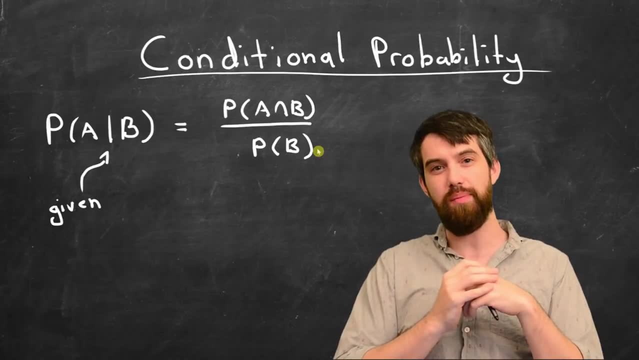 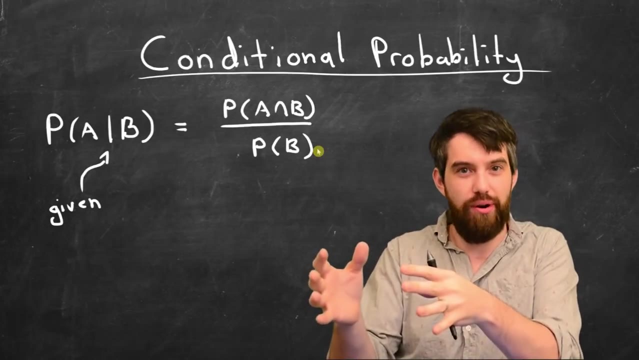 of A occurring given B. So the sort of sum total of all the possibilities are going to be: whatever the possibility is, B is going to be, because we know that B has occurred. But then we're asking: well, how often is it likely the case that you have A and B occurring amongst all the possibilities? 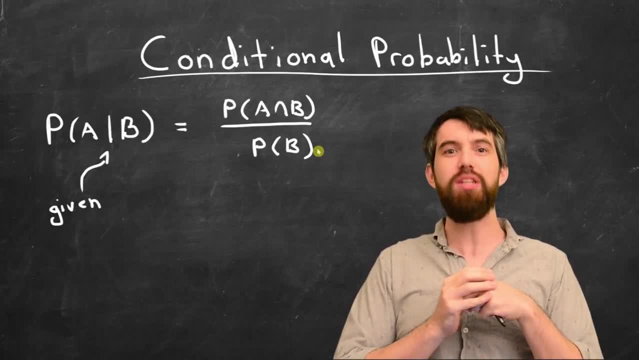 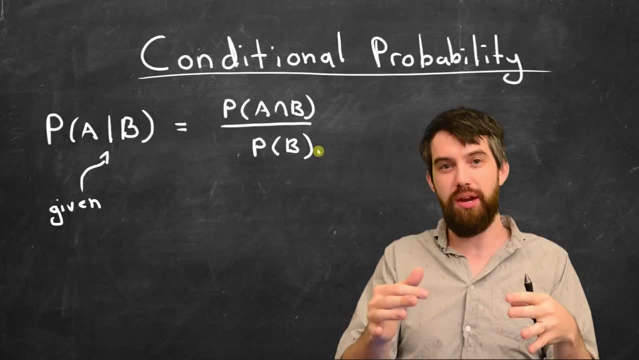 where B occurs. So that's why we have this formula. This is what is the probability that A and B occurs. That's the numerator divided by all the possible ways that B could occur. That's the denominator. Note that in most cases, if we're just talking about non-conditional probabilities, 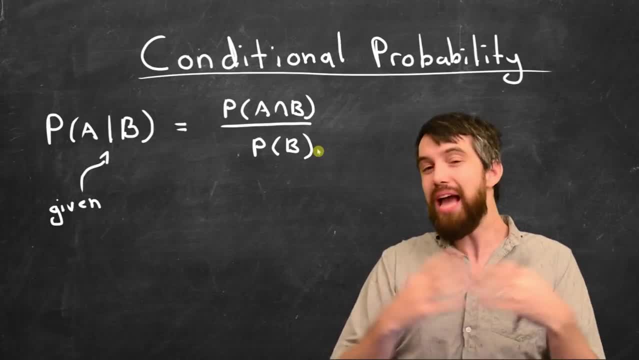 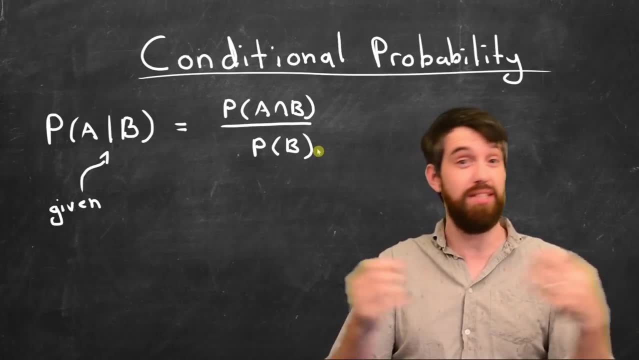 but the probability of A is without any other information. we actually are typically dividing by something the same way, It's just that we divide by the probability of all possible events the entire sample space, the entire universe of possibilities, which is just one. 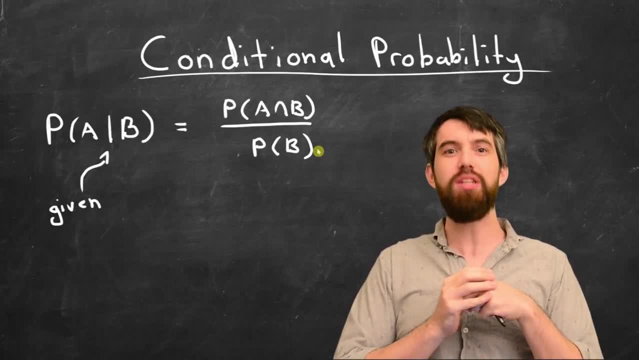 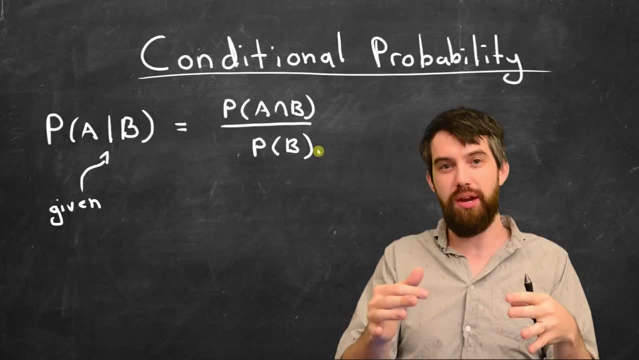 where B occurs. So that's why we have this formula. This is what is the probability that A and B occurs. That's the numerator divided by all the possible ways that B could occur. That's the denominator. Note that in most cases, if we're just talking about non-conditional probabilities, 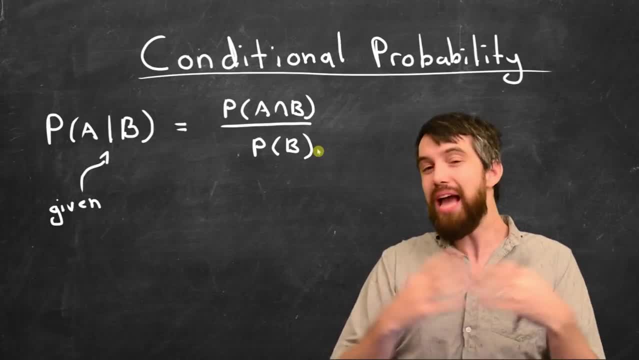 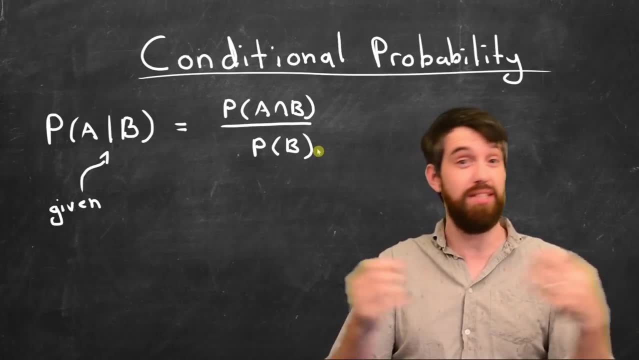 but the probability of A is without any other information. we actually are typically dividing by something the same way, It's just that we divide by the probability of all possible events the entire sample space, the entire universe of possibilities, which is just one. 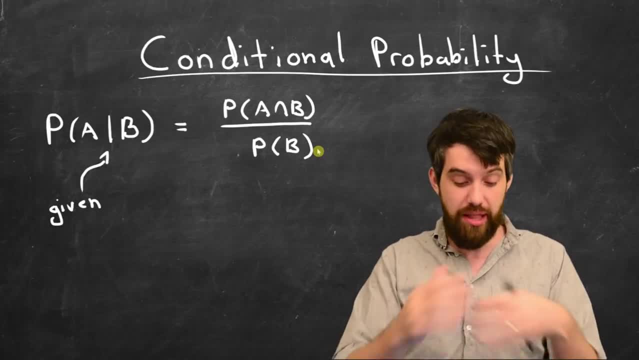 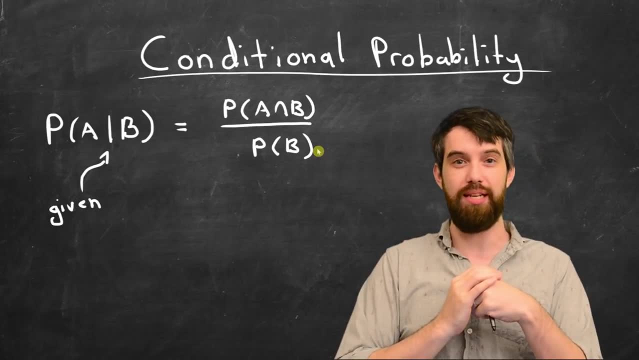 So we are in fact always dividing out by something. In the case of conditional probability, it's that we're dividing out by the probability of B, the thing that we're told has to exist. Now we can sort of visualize how this is going to work by using a Venn diagram. 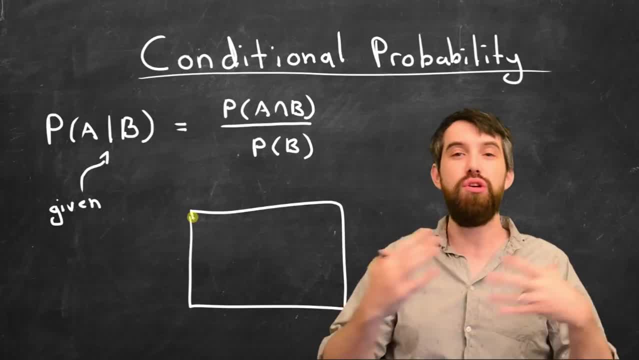 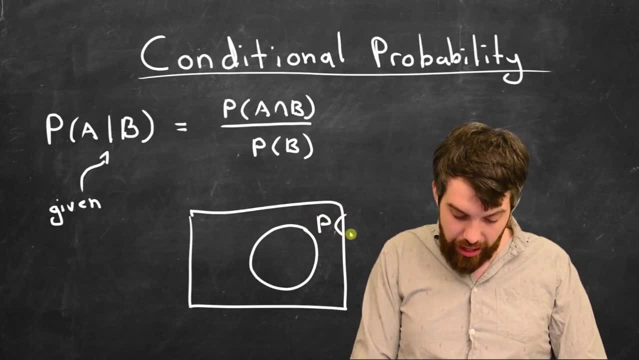 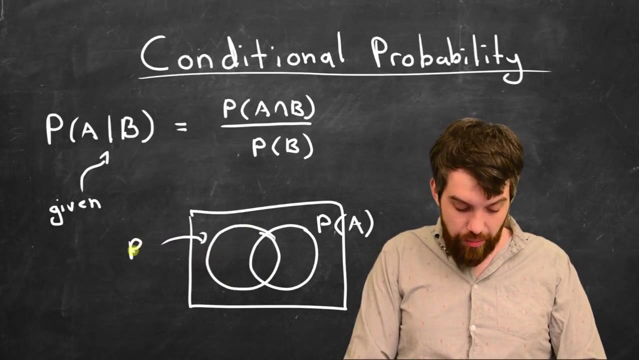 So a Venn diagram. I'm going to list my entire universe of possibilities and then I can say that, look, I have within my entire universe some probability of an event A occurring and I can also have a probability of some event B occurring. Well, if I'm looking at this sort of conditional 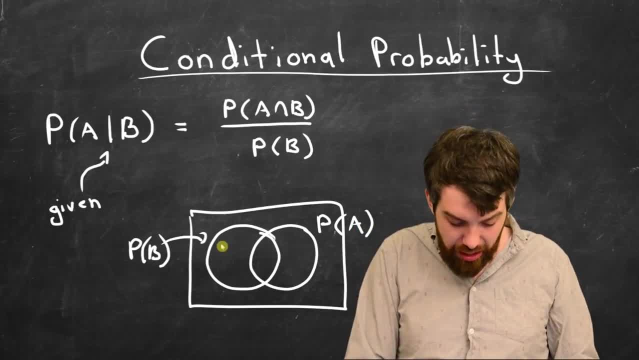 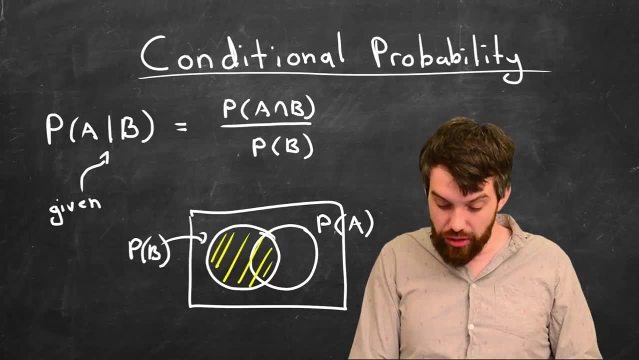 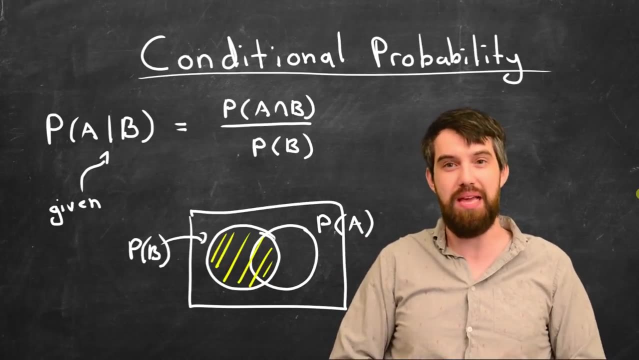 probability. Well, conditional probability is saying: look, I'm in the scenario where this event B is occurring. I'm assuming that event B occurs, And then what I'm really interested in is: what is the probability of this event A occurring, given that I'm in this event B and 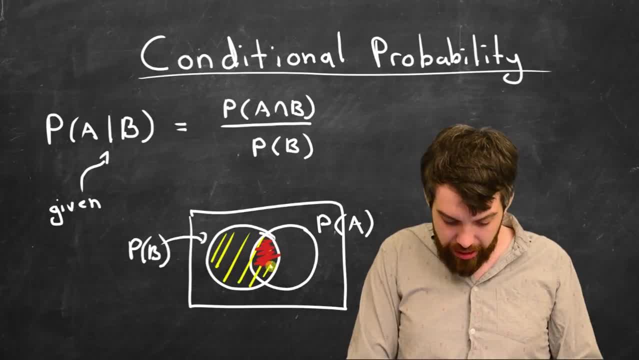 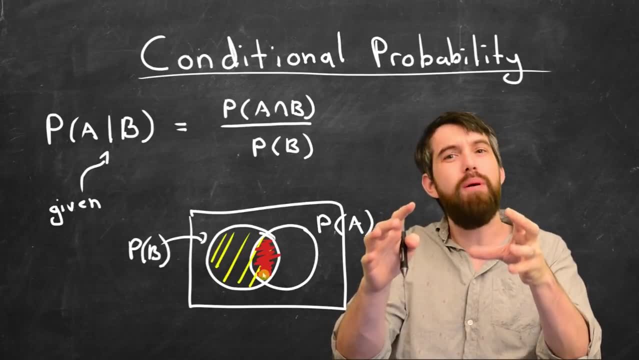 event B has occurred, In which case I'm really interested in this intersection here. In other words, I care about this ratio of the probability of the intersection to the probability of B occurring. the red divided out by the yellow here. Now, in this example, I've given you something. 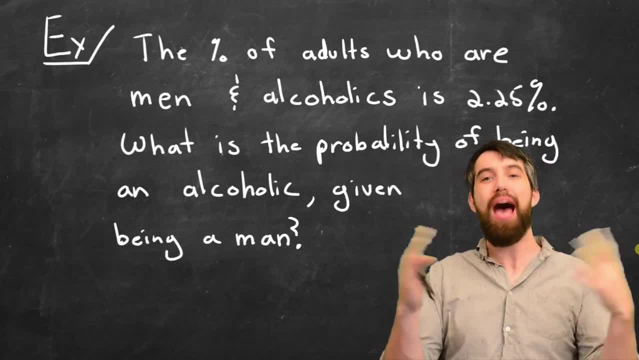 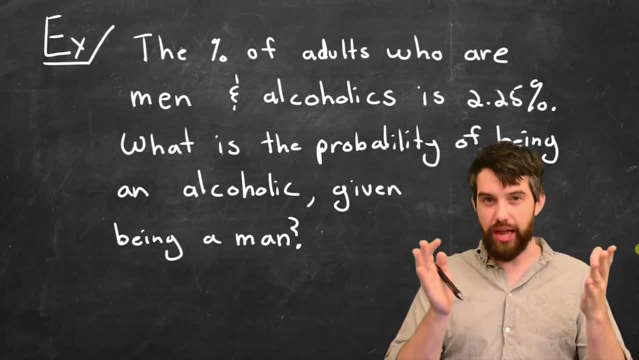 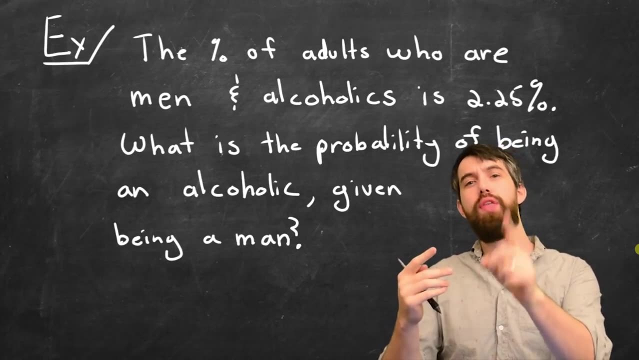 I've given you an intersection. I've told you that the percent of adults who are both male and who are alcoholics is going to be- it looks like- 2.25 percent. I had to look this up. And then the question is: what is the probability that you're an alcoholic if you know that you're? 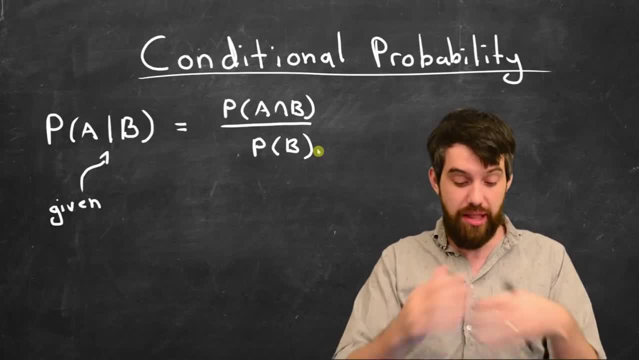 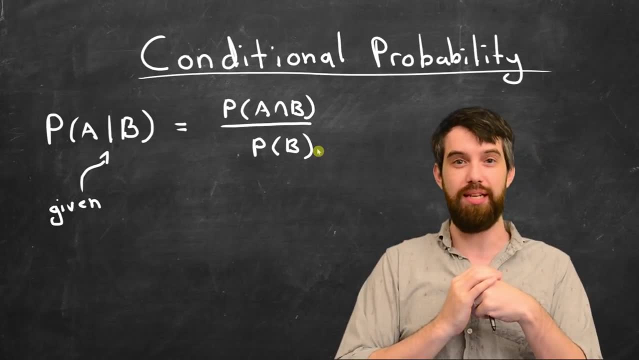 So we are in fact always dividing out by something. In the case of conditional probability, it's that we're dividing out by the probability of B, the thing that we're told has to exist. Now we can sort of visualize how this is going to work by using a venn diagram. So 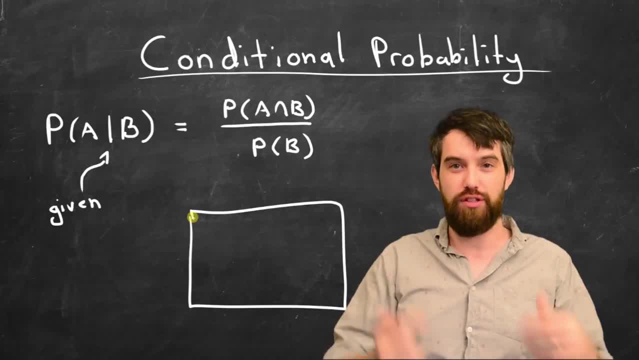 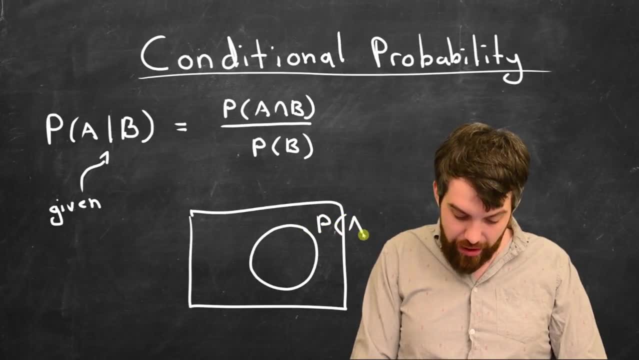 a venn diagram. I'm going to list my entire universe of possibilities and then I can say that look, Within my entire universe, I can have some probability of an event A occurring. I could also have a probability of some event B occurring. Well, if I'm looking at this sort of 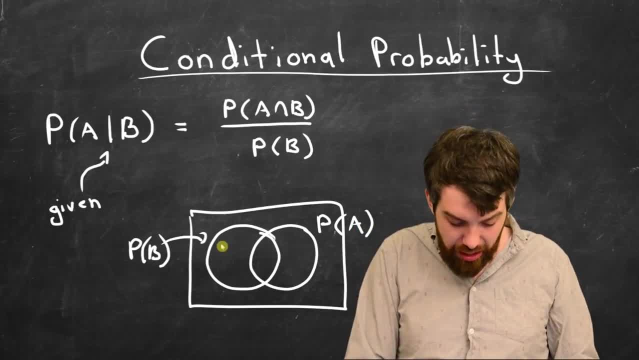 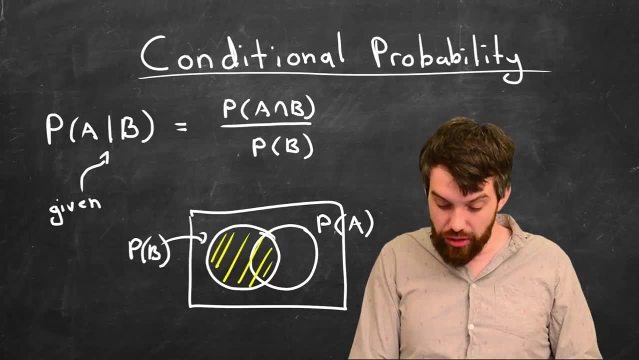 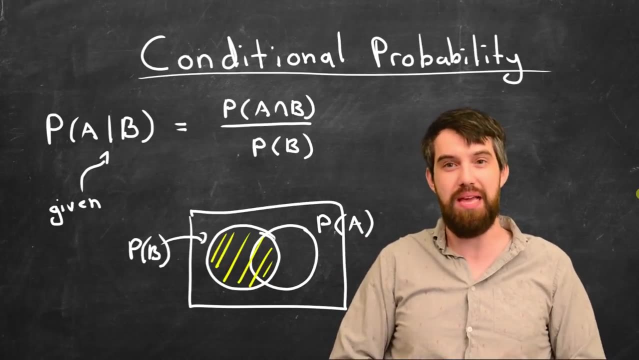 probability. Well, conditional probability is saying: look, I'm in the scenario where this event B is occurring. I'm assuming that event B occurs, And then what I'm really interested in is: what is the probability of this event A occurring, given that I'm in this event B and 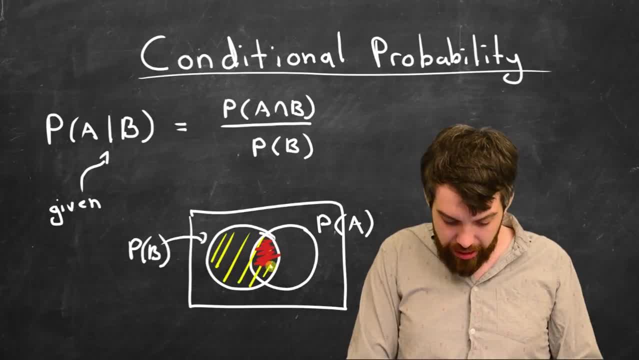 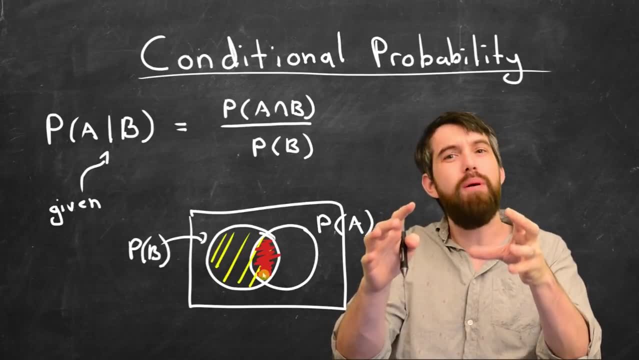 event B has occurred, In which case I'm really interested in this intersection here. In other words, I care about this ratio of the probability of the intersection to the probability of B occurring. the red divided out by the yellow here. Now, in this example, I've given you something. 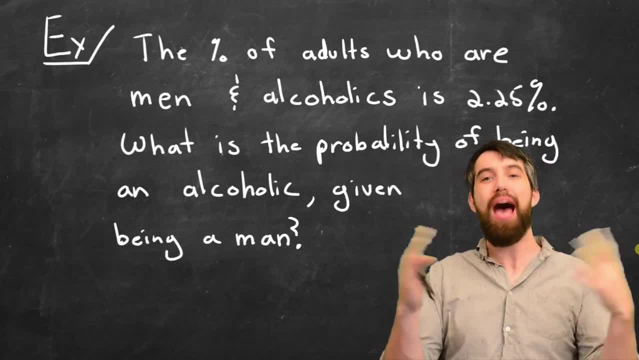 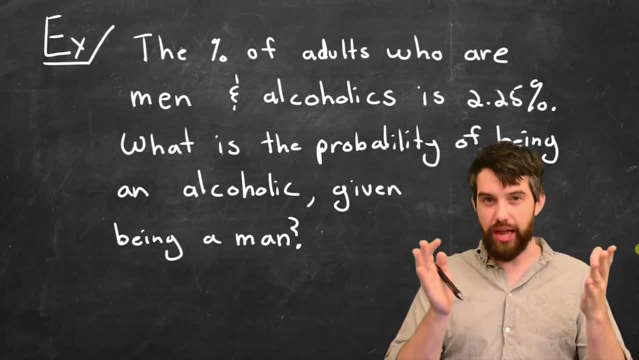 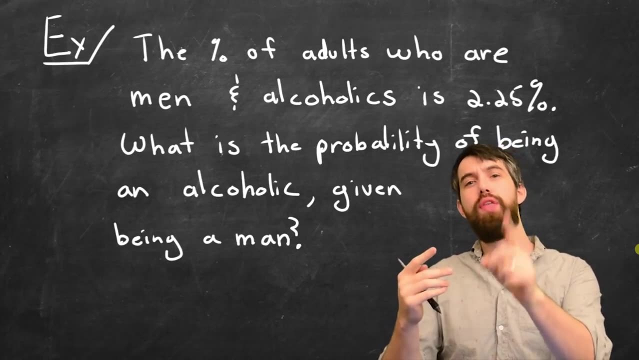 I've given you an intersection. I've told you that the percent of adults who are both male and who are alcoholics is going to be- it looks like- 2.25 percent. I had to look this up. And then the question is: what is the probability that you're an alcoholic if you know that you're? 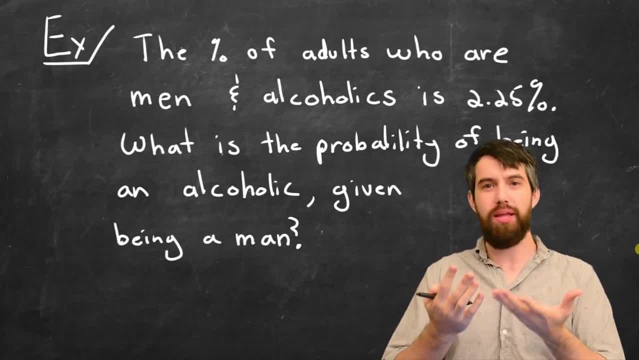 a male, We can look at what the probability of being an alcoholic is in general, but I'm interested in this problem. It's: if you know that your patient is a male, what is the probability that they're an alcoholic? So we're going to use conditional probability to figure this out, because we know something. 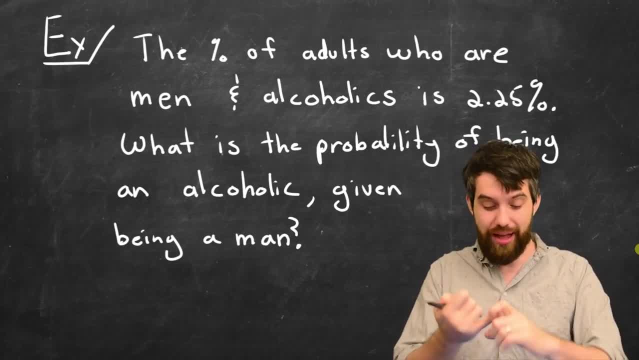 about the intersection, the probability of being an alcoholic and a male. that's 2.25 percent. We know what the probability of being a male is. I'll approximate it at 50 percent And we can use those two facts together to get the conditional probability, the probability that you're an. 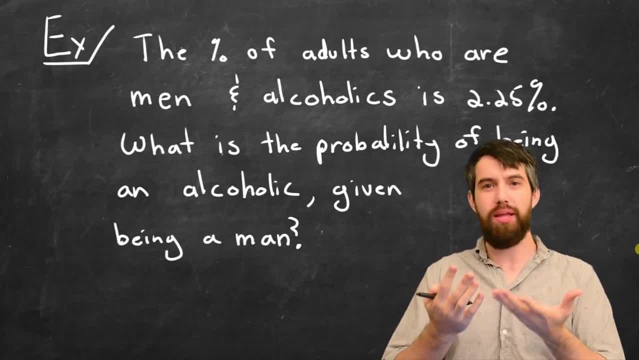 a male, We can look at what the probability of being an alcoholic is in general, but I'm interested in this problem. It's: if you know that your patient is a male, what is the probability that they're an alcoholic? So we're going to use conditional probability to figure this out, because we know something. 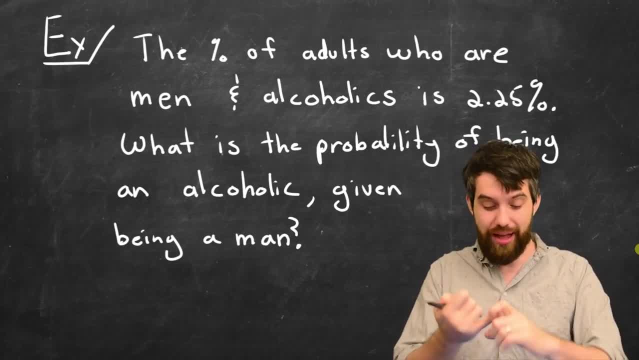 about the intersection, the probability of being an alcoholic and a male. that's 2.25 percent. We know what the probability of being a male is. I'll approximate it at 50 percent And we can use those two facts together to get the conditional probability, the probability that you're an. 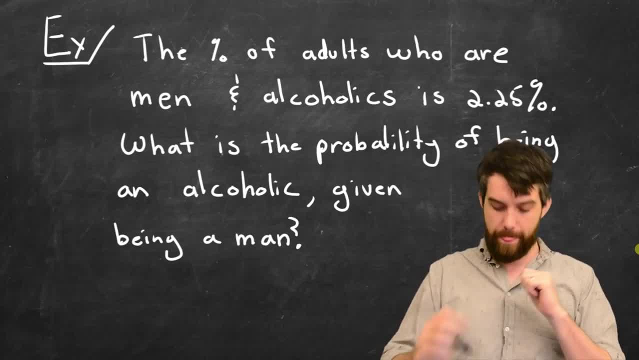 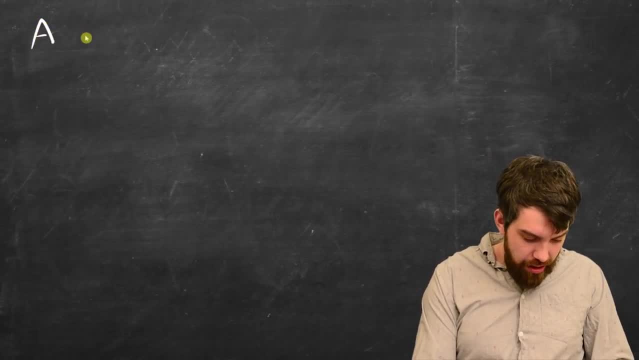 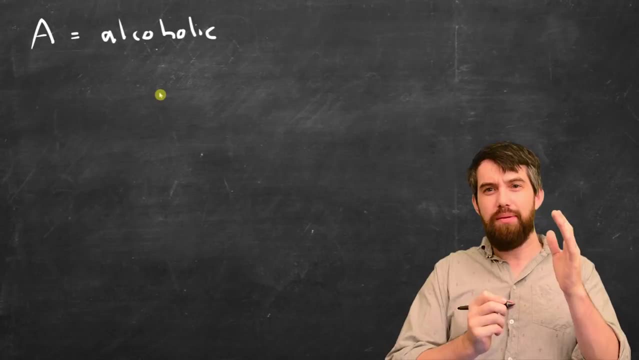 alcoholic, given that you're an adult male. Now I need to define a little bit of a sort of notation before I plug it into my formula. I'm going to let a- this is going to be equal to the particular event of being an alcoholic, And then I'm going to let b. 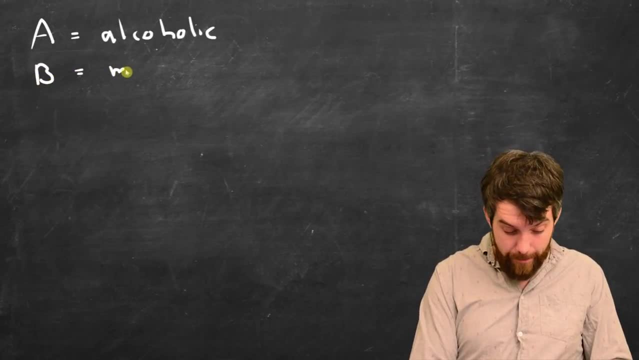 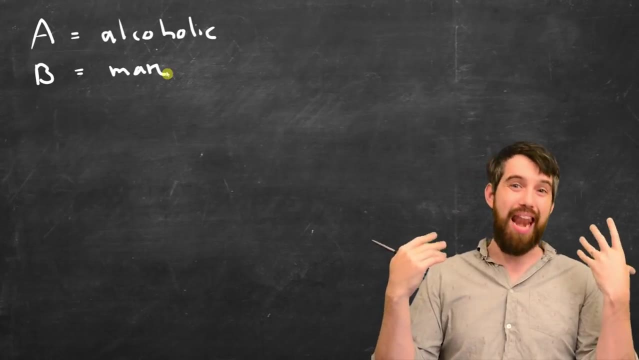 be the event that you're going to be a man. So there's two different things we can do. that's what's the probability of being an alcoholic. that's the probability of being a man. what's the probability of being an alcoholic and a man. That's the thing that. 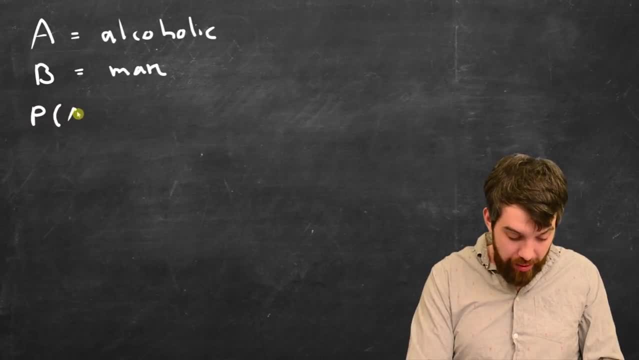 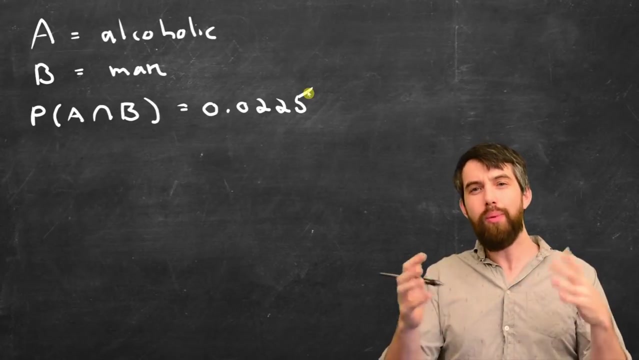 we were given. We were given, in particular, that the probability of being an alcoholic and being a man, that this was equal to 0.0225, or in other words, two and a quarter percent. and so what we're really asking when i ask: what is the probability that you're an alcoholic? 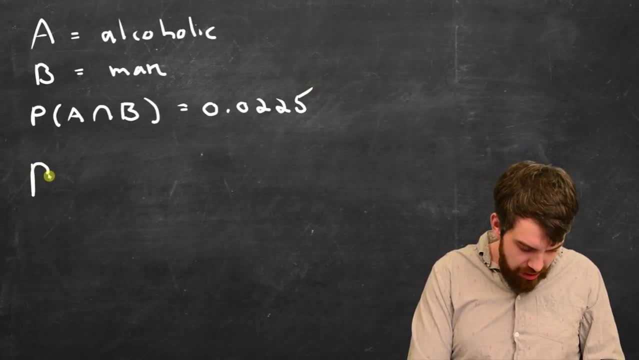 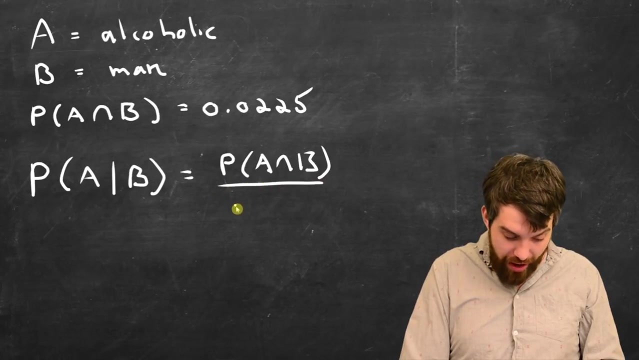 given that you're a man, is we're asking what is the probability of being a being an alcoholic, given that you're a man, and- and we know that from our formula, this is going to be the probability of a intersect b, so the probability of being both all divided by the probability 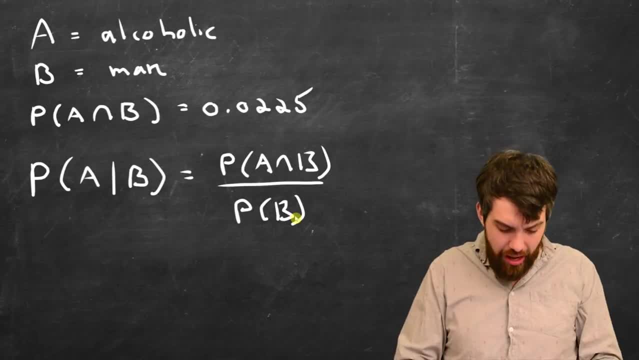 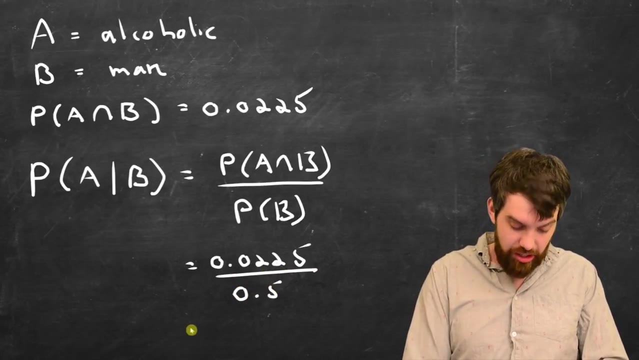 of just b, in other words the probability of being a man, and we know these two different answers. the top is going to be 0.0225, and then i'm going to be dividing this by the probability of a man and i'm going to say that that's 0.5. i'm going to assume it's exactly 50 percent and therefore 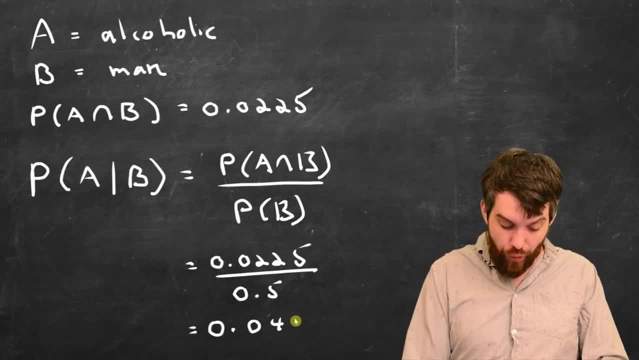 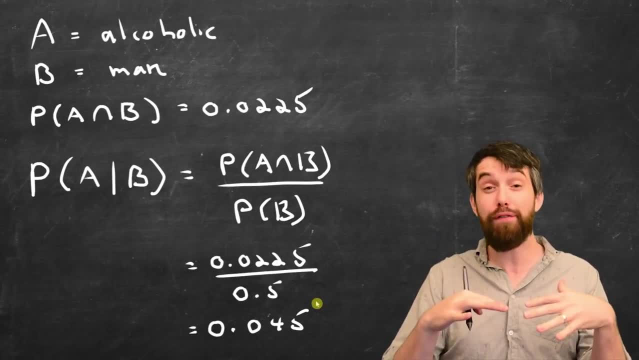 what i'm going to get is 0.04, 0.04, 0.04. five or about four and a half percent for adult males. by the way, it's a little bit smaller for adult females. it's about two and a half percent for adult females. so this is a way that we've 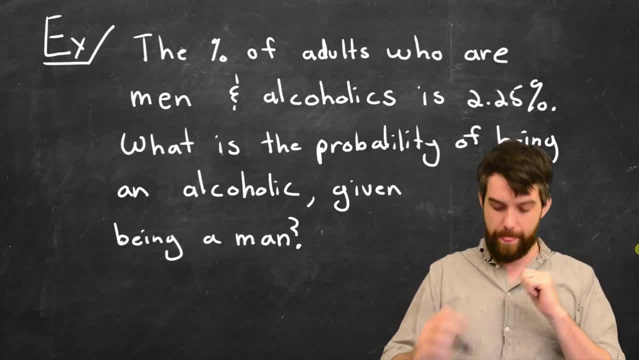 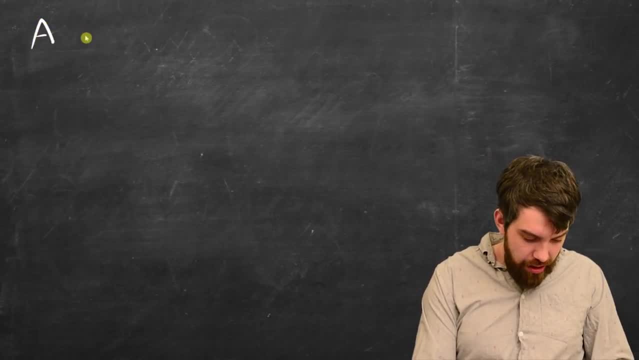 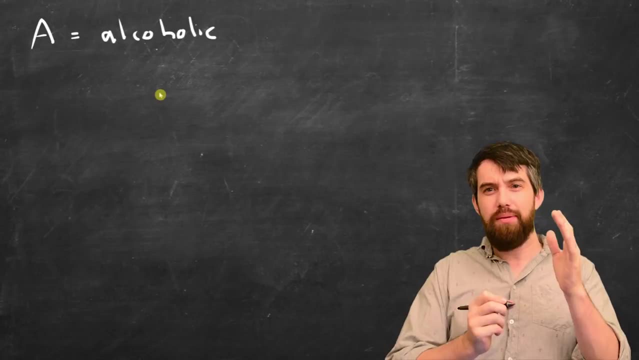 alcoholic, given that you're an adult male. Now I need to define a little bit of a little bit of notation before I plug it into my formula. I'm going to let a. this is going to be equal to the particular event of being an alcoholic, And then I'm going 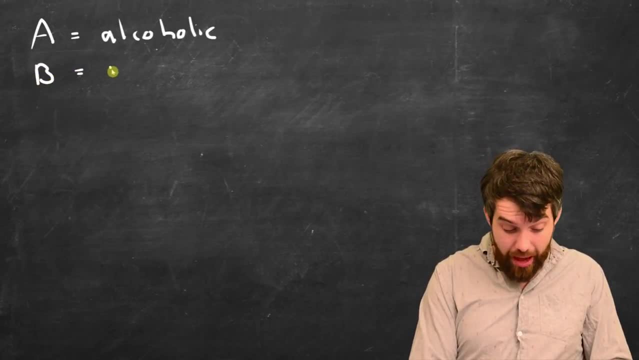 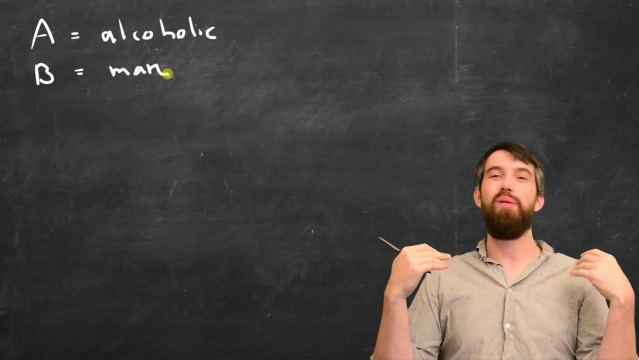 to let b be the event that you're going to be a man. So there's two different things we can do. We can ask: what's the probability of being an alcoholic, What's the probability of being a man, What's the probability of being an alcoholic and a man? That's the thing. 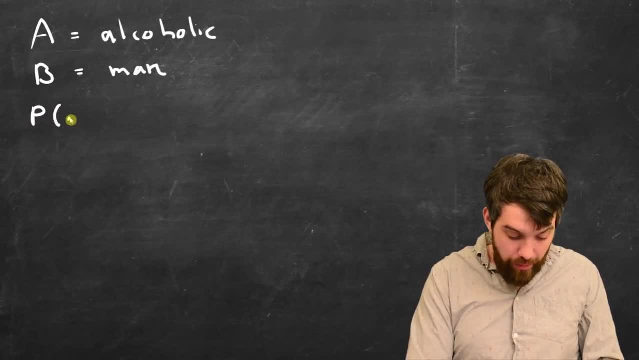 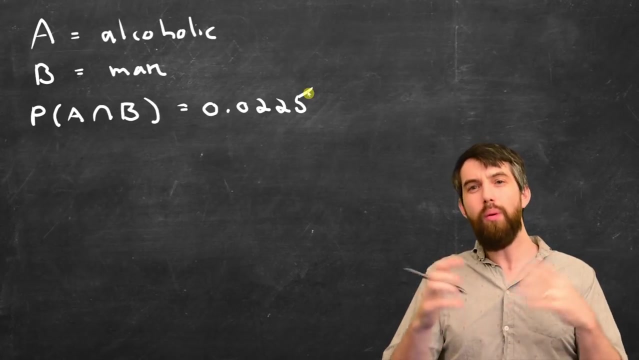 that we were given. We were given, in particular, that the probability of being an alcoholic- alcoholic- and being a man, that this was equal to 0.0225, or, in other words, two and a quarter percent. And so what we're really asking when I ask: what is the probability that you're an alcoholic? 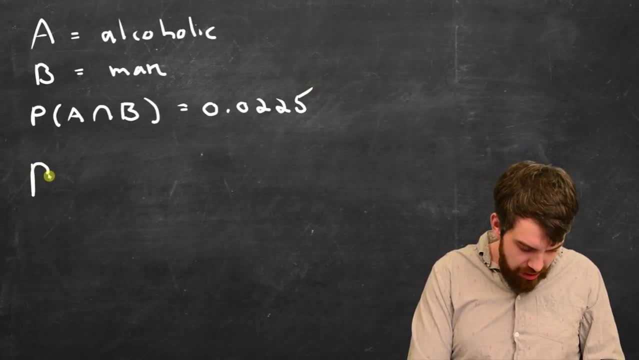 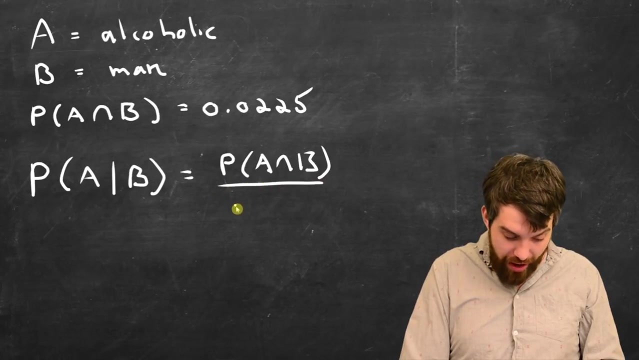 given that you're a man, is we're asking what is the probability of being A being an alcoholic, given that you're a man, And we know that from our formula, this is going to be the probability of A intersect B, So the probability of being both all divided by the probability 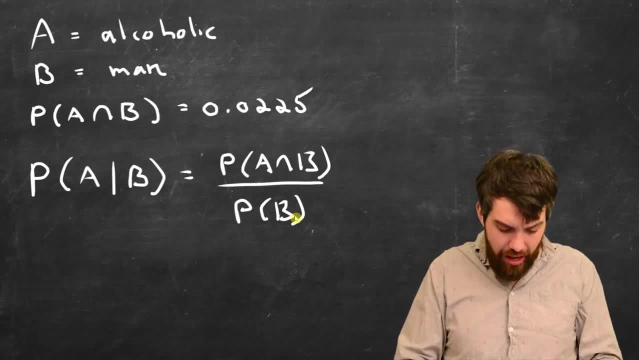 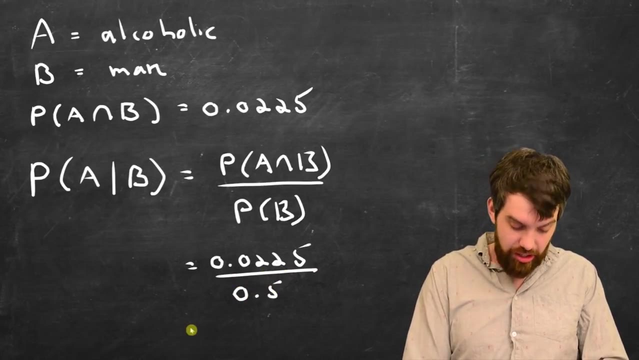 of just B, In other words the probability of being a man, And we know these two different answers- The top is going to be 0.0225.. And then I'm going to be dividing this by the probability of a man And I'm going to say that that's 0.5.. I'm going to assume it's exactly 50%. 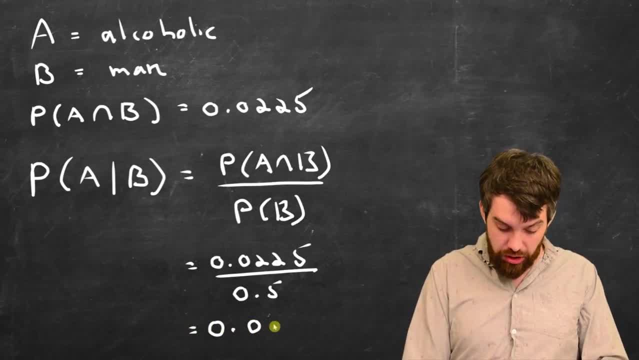 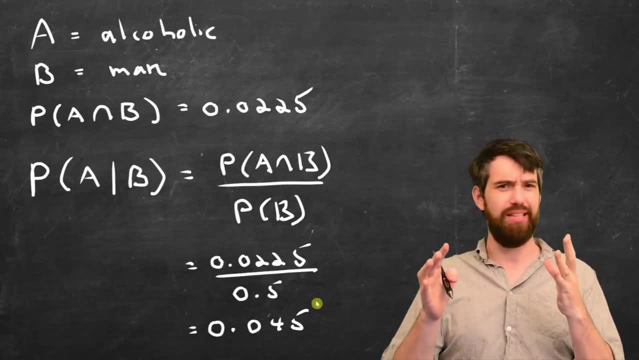 And therefore what I'm going to get is 0.0425.. 0.0425 is going to be the probability of being an alcoholic. given that you're a man, By the way, it's a little bit smaller for adult females: It's about two and a half percent. for. 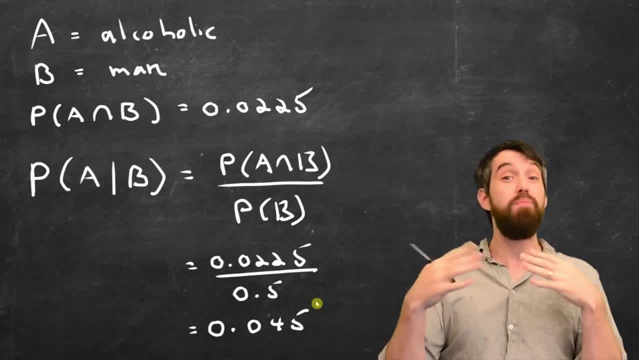 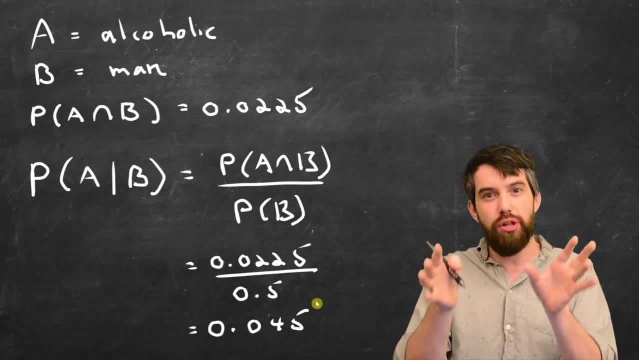 adult females. So this is a way that we've been able to compute this result- the probability of being an alcoholic, given that you're a male, via this technique of conditional probability.